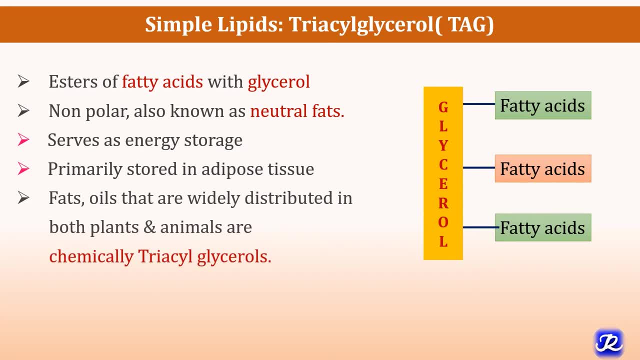 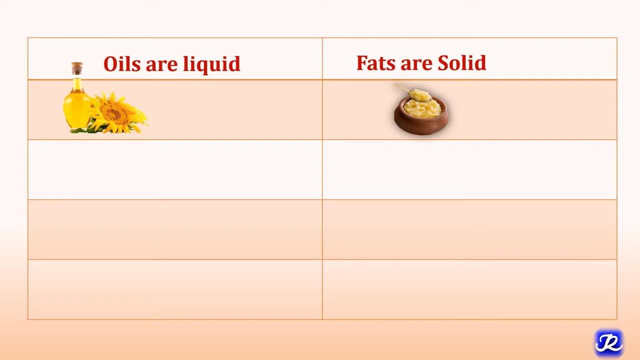 oils that are widely distributed in both plants and animals. These amino acids are chemically triacylglycerol. The difference between fats and oils is only physical. In the oils, high proportion of unsaturated and short chain fatty acids are present, While fats, which are solid in nature, high precautions of saturated and long chain. 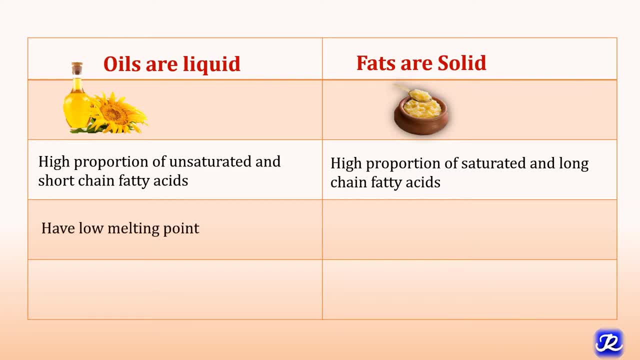 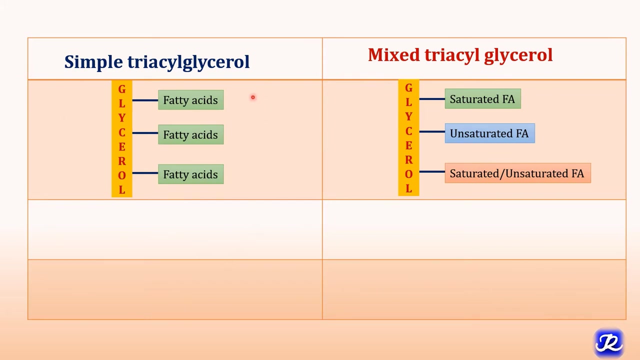 fatty acids are present. Oil have those multiple melting points and fats have high melting point. Oils are generally of vegetable origin, like sunflower oil, soya bean oil, and fats are mainly of animal origin, for example ghee. A triacylglycerol is called as simple triacylglycerol when all the fatty acid attached to the glycerol backbone are same. 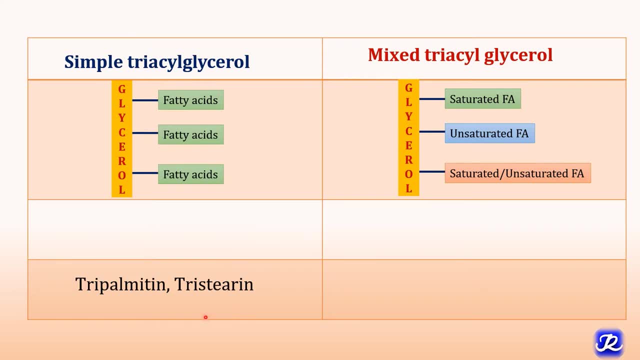 For example tripamidine and triasteirine. In case of mixed triacylglycerol, the first fatty acid can be saturated fatty acid. the second fatty acid attached to glycerol backbone is mostly unsaturated fatty acid, and the third fatty acid is either saturated or unsaturated fatty acid. 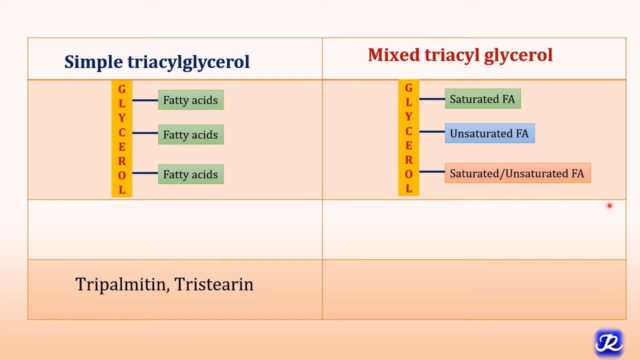 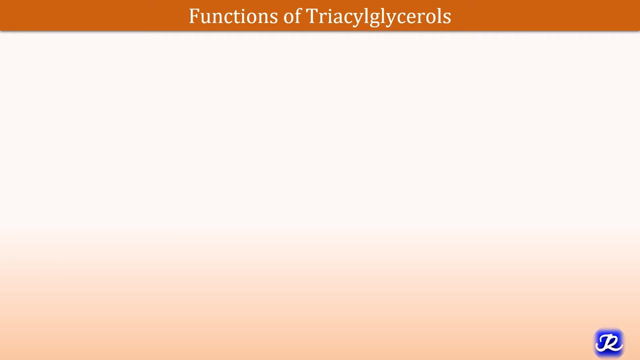 It is the mix of both saturated and unsaturated fatty acid, and that's why it is called as mixed triacylglycerol Animal fats. Animal fats contain more saturated fatty acids, and vegetable fats contain more unsaturated fatty acids. The most important function of triacylglycerol is storage of energy in adipose tissue. 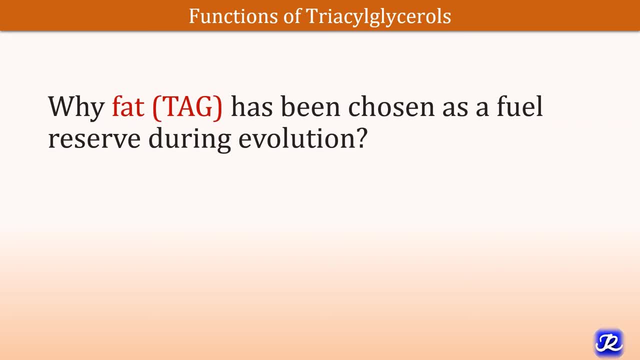 Now the important question is why fat ie TAG has been chosen as a fuel reserve during evolution, Because we know that triacylglycerol stores allow survival for several weeks. Why, While the carbohydrate form of energy storage, ie glycogen, it sustains physiological function for about 24 hours. 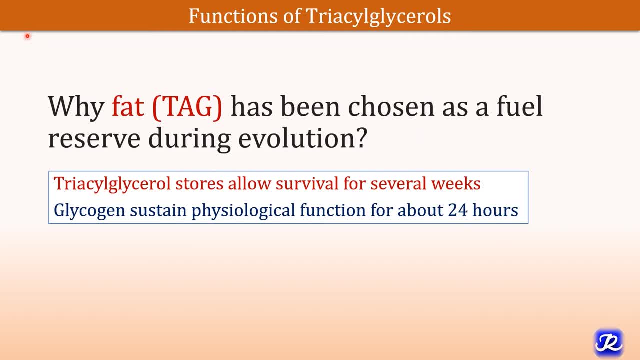 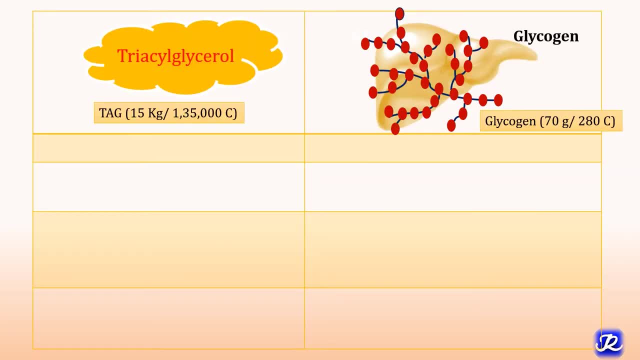 So why the nature has chosen this triacylglycerol as a fuel reserve? Let's try to understand the answer of this question. Triacylglycerol is a form of energy storage in case of lipids, and glycogen is a form of energy storage in case of carbohydrates. 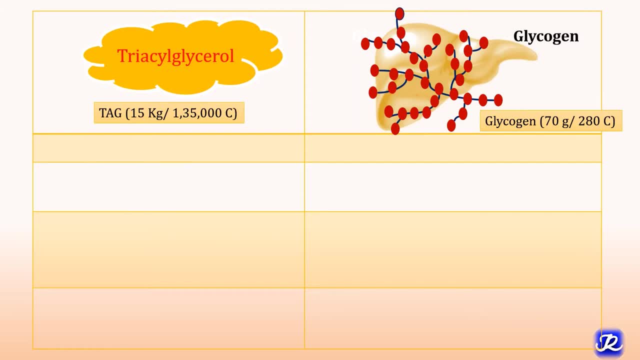 Triacylglycerol is stored in the adipose tissue and glycogen is stored in the lipids And glycogen is stored in the liver. TAG is nonpolar and hydrophobic, while glycogen is more polar. TAG is stored in anhydrous form. 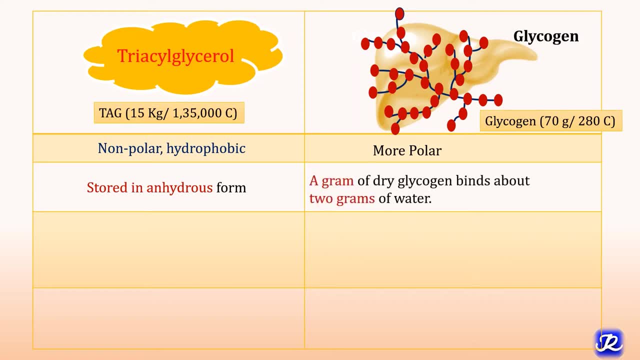 It does not require water for its storage, while glycogen requires water. A gram of dry glycogen requires 2 grams of water for its storage, And a gram of anhydrous fat stores more than 6 times as much energy as a gram of hydrated glycogen. 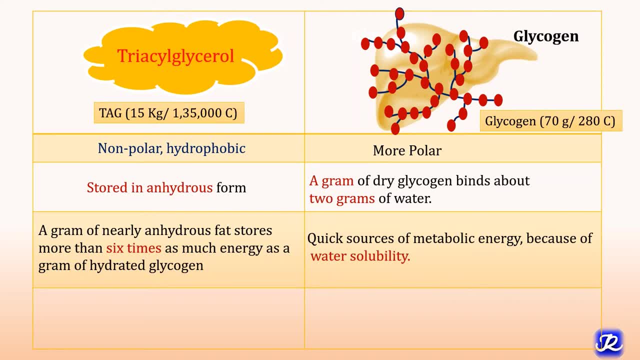 But the glycogen is not a hydrophobic. Glycogen is a quick source of metabolic energy because of its water solubility. It is a highly concentrated form of energy, that is, TAG is highly concentrated. It produces 9 kilocalories per gram on oxidation, while glycogen breakdown produce only 4 kilocalories per gram. 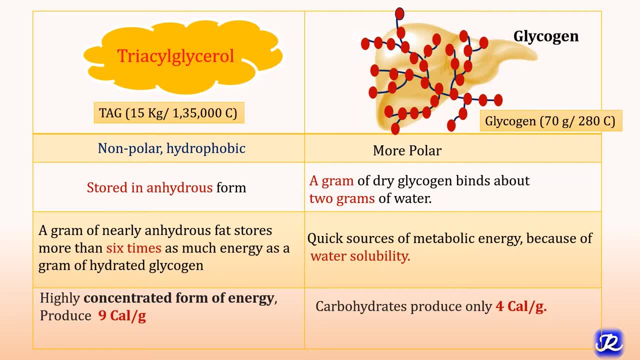 There are two main reasons for fat being the major fuel reserve of the body. The first is that TAG are highly concentrated form of energy, producing 9 kilocalories per gram on oxidation, as compared to carbohydrates, which produces just 4 kilocalories per gram. 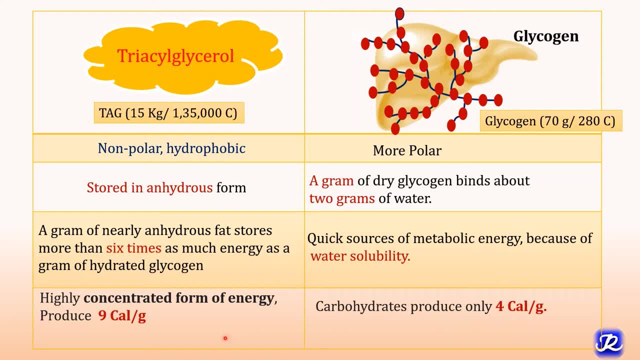 And this is because the fatty acids in TG are in reduced form. And the second reason is that TAG does not require water for its storage and glycogen requires water for its storage. 1 gram of glycogen requires 2 gram of water And we know that in a healthy individual of 70 kg, about 15 kg triacylglycerol are stored in the adipose tissue, which is equivalent to 1,35,000 kilocalories. 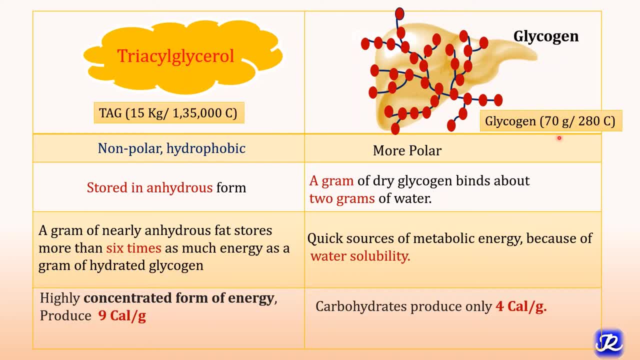 And glycogen storage is just 70 to 80 gram, which is equivalent to 280 kilocalories. Now imagine if this much of energy- like, for example, 15 kg energy, were to be stored as glycogen Instead of fat. then it requires so much of water that the weight of person would increase by at least 55 kg, and this explains why fat has been chosen as a fuel reserve during evolution. 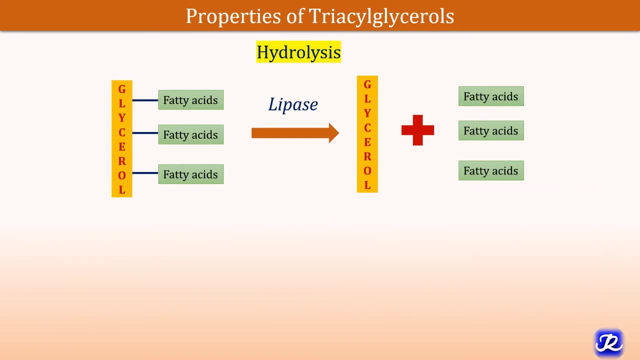 Now let's talk about the properties of triacylglycerol, and the first is hydrolysis. Triacylglycerol undergoes stepwise enzymatic hydrolysis to finally liberate free fatty acids and glycerol, And this process of hydrolysis is catalyzed by enzymes, lipases. 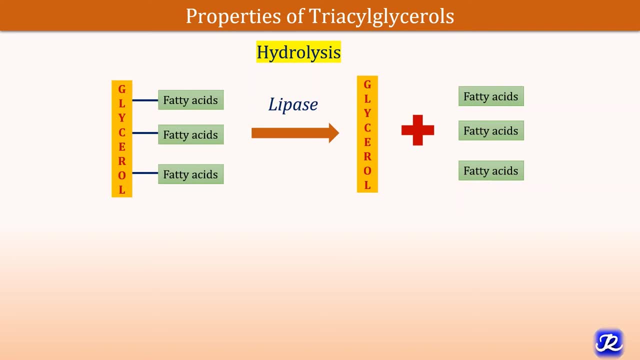 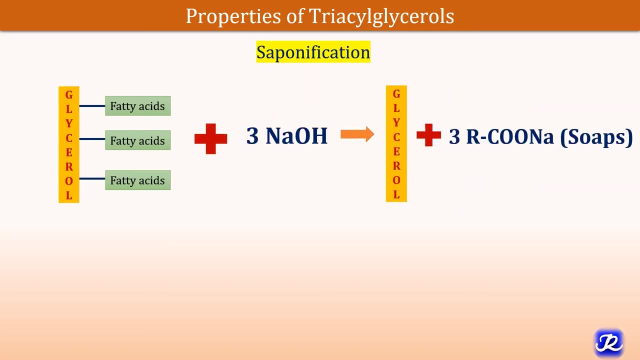 And this process is important for digestion of fat in the gastrointestinal tract and fat mobilization from the adipose tissue. Second property of triacylglycerol is saponification. It is the hydrolysis of triacylglycerol by alkali to produce glycerol and soaps. 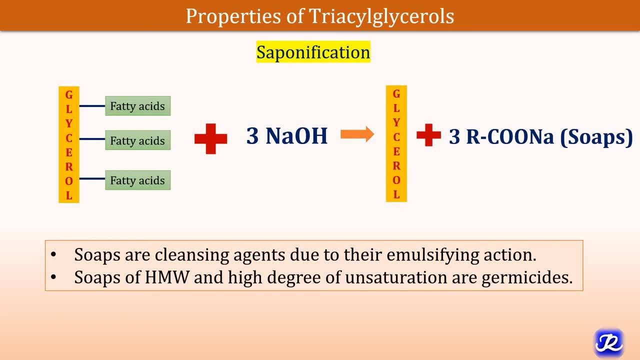 Soaps are cleansing agent. due to their emulsifying action, Soaps of high molecular weight and high degree of unsaturation are germicides. Soaps molecule kills corona virus by disrupting the fatty layer or pores surrounding the virus. Hydrogenation is the property of triacylglycerol. 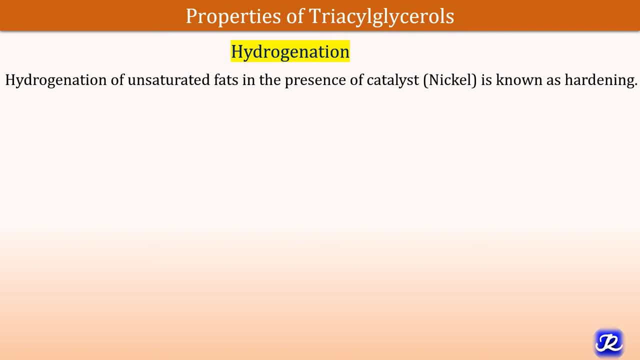 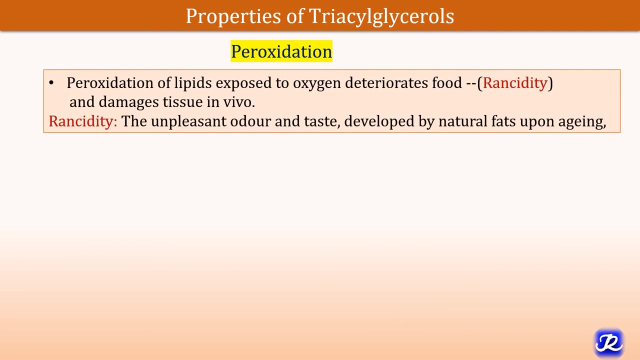 Hydrogenation of unsaturated fats in the presence of some catalyst is known as glycerol. Liquid fats of plant origin are converted into solid fats by hydrogenation, for example margarine and vegetable ghee. Peroxidation of lipids exposed to oxygen deteriorates food, which is called as rancidity. 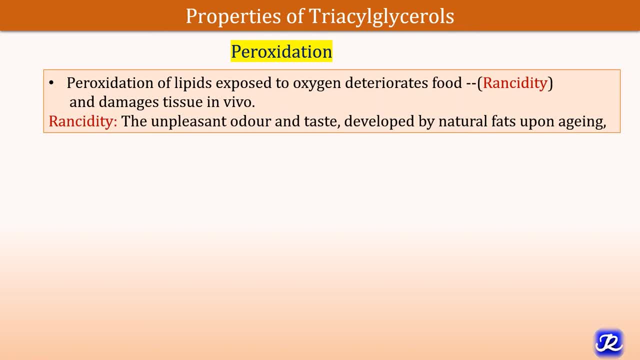 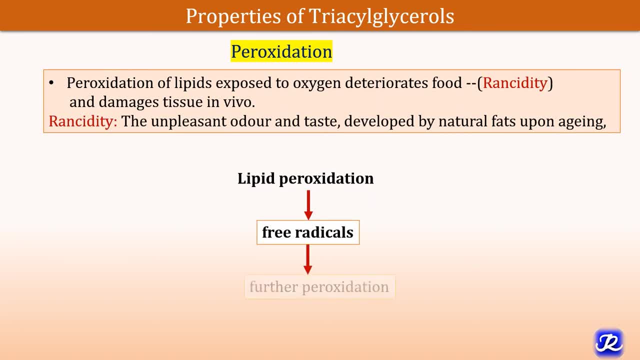 Lipid peroxidation is like a chain reaction which produces free radicals and further it causes peroxidation Over heating and repeated heating of oil leads to libid peroxidation. Antioxidantsát 확인ize vitamin E. Antioxidants like vitamin E are added. 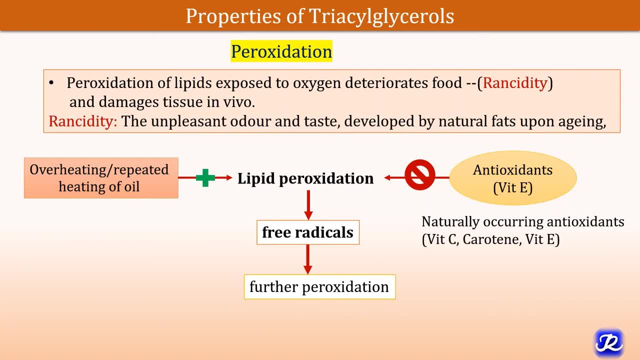 There are certain natural antiaging products, including Howie你需要 occurring antioxidants like vitamin E, vitamin C, carotene and some food additives are also antioxidants, like butylated hydroxy anisole, that is, BHA, and butylated hydroxy toluene, like DHT.